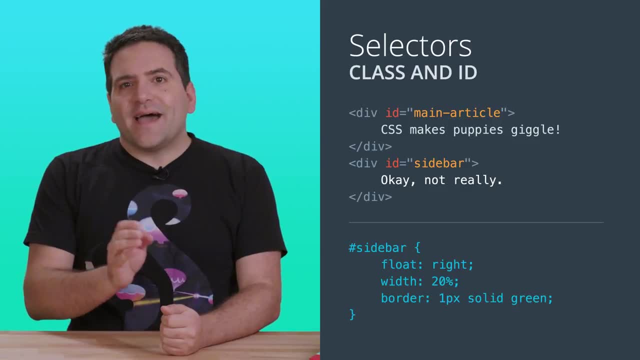 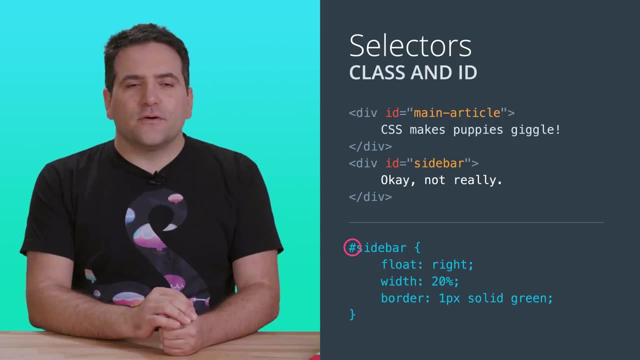 You just make them up. But to apply a style to elements by id, instead of a dot in the selector you put a hash mark or a number sign or one of these things. anyway, 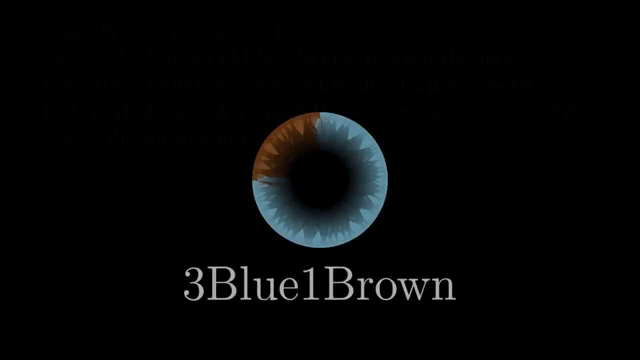 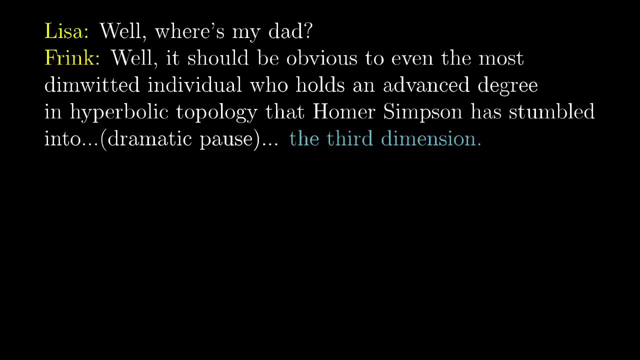 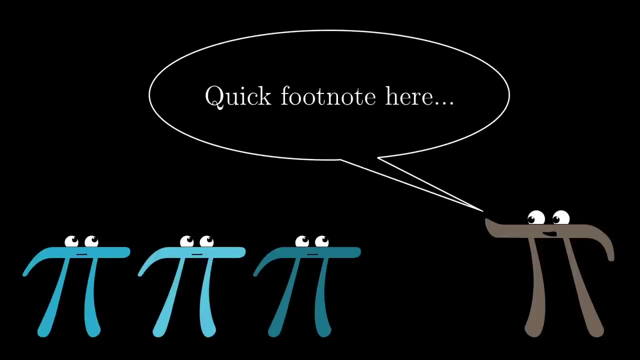 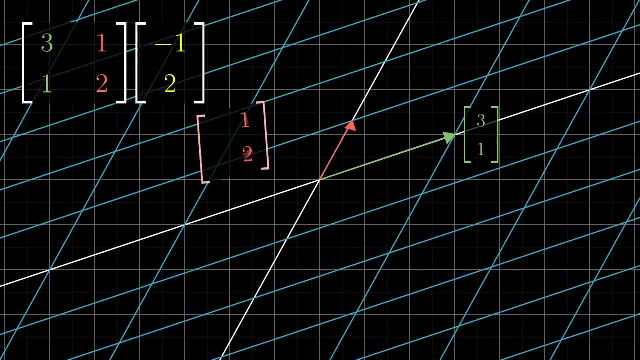 Hey folks, I've got a relatively quick video for you today, just sort of a footnote between chapters. In the last two videos I talked about linear transformations and matrices, but I only showed the specific case of transformations that take two-dimensional vectors to other. 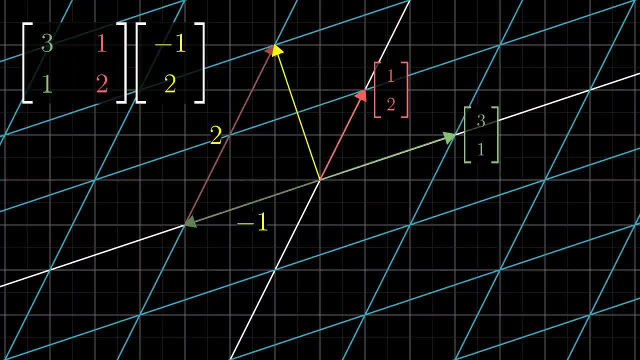 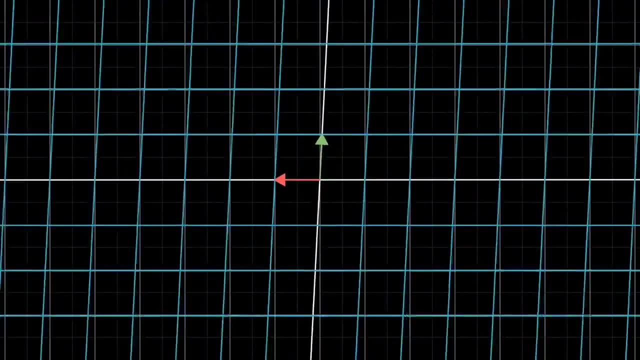 two-dimensional vectors In general. throughout this series we'll work mainly in two dimensions, mostly because it's easier to actually see on the screen and wrap your mind around. But more importantly than that, once you get all the core ideas in two dimensions, they carry. 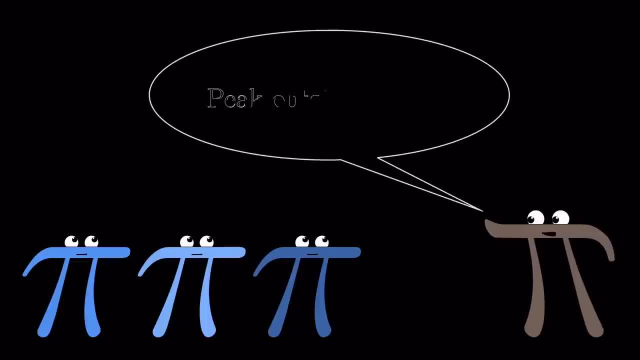 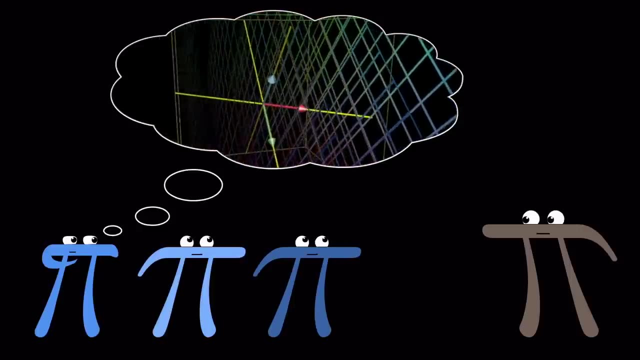 over pretty seamlessly to higher dimensions. Nevertheless, it's good to peek our heads outside of Flatland now and then. to you know see what it means to apply these ideas in more than just those two dimensions. For example, consider a linear transformation with three-dimensional. 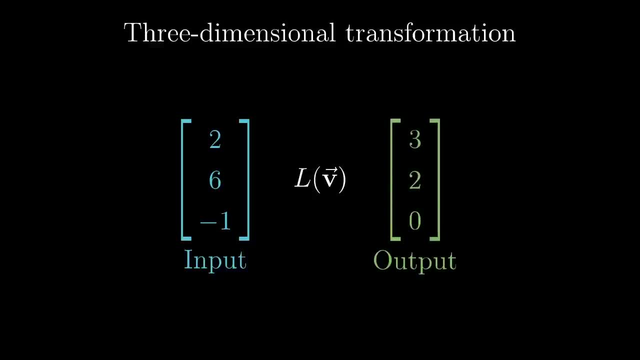 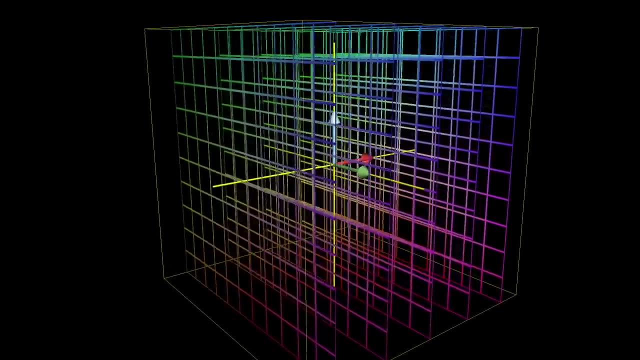 vectors as inputs and three-dimensional vectors as outputs. We can visualize this by smooshing around all the points in three-dimensional space, as represented by a grid, in such a way that keeps the grid lines parallel and evenly spaced and which fixes the origin. 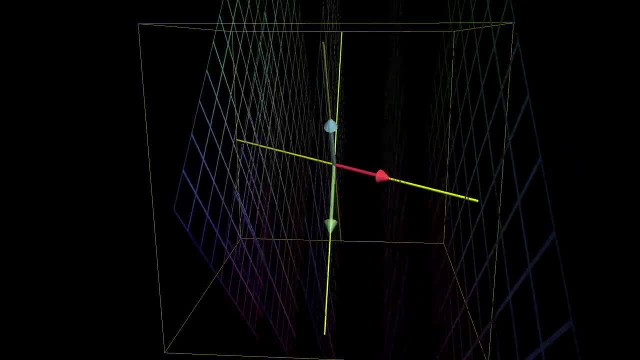 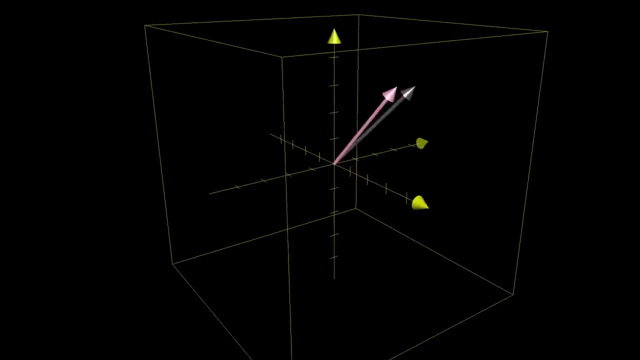 in place And, just as with two dimensions, every point of space that we see moving around is really just a proxy for a vector who has its tip at that point, and what we're really doing is thinking about input vectors moving over two dimensions.